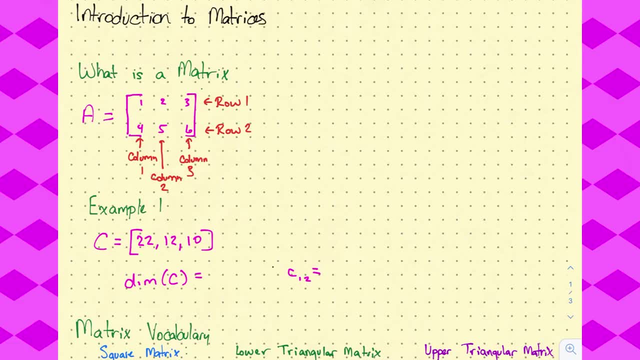 statistical data with numbers, but also graphical data with pictures. The following is an example of a matrix. This matrix, A, has two rows and three columns, so we would call A a 2 by 3 matrix. This is the dimension of the matrix If M and N are positive integers. 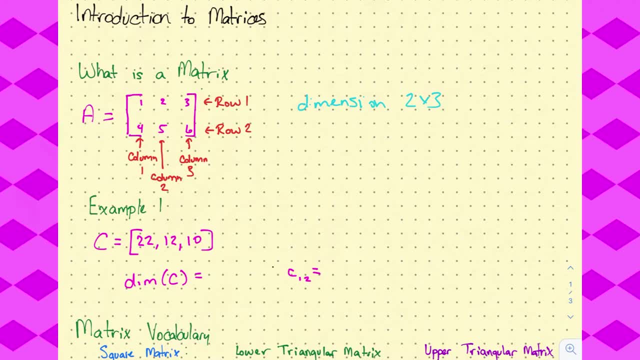 then we say an M by N matrix has M rows and N columns. Whenever we list the dimensions of a matrix- first it's important it's always rows and then columns. We use a similar naming scheme when we talk about each element or each entry in a matrix. For example, A 1, 2,. these are subscripts. 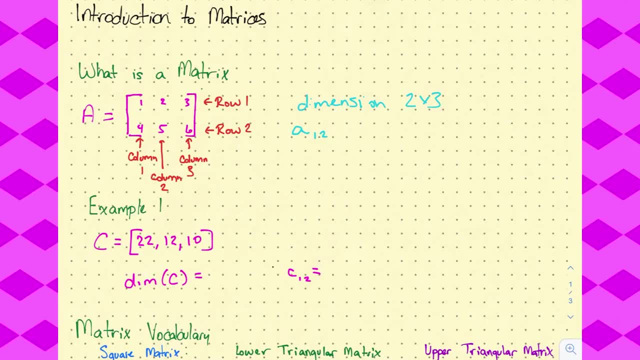 these subscripts define the location. So A 1- 2 refers to the element in the first row, second column. A 1- 2 is the element 2.. So here's an example: Matrix C is 22,, 12,, 10.. This matrix has one. row and three columns. Therefore, if A 1- 2 is the element in the second row, then A 1- 2 is 12, 2.. If A 1- 2 is the element in the second row, then A 1- 2 is the element in the second row. This matrix has one row and two columns. 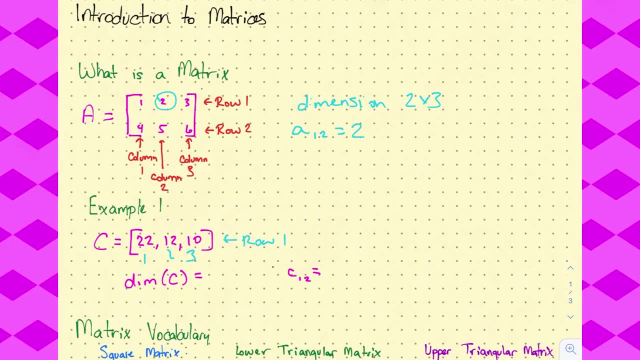 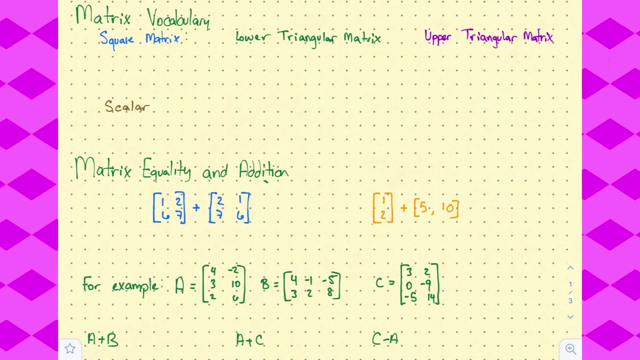 So we would say this matrix is a 1 by 3 matrix. So if I want to know what element C12 is, I go to the first row, second column. C12 is equal to 12.. There are a few specific terms with matrices that we need to define. 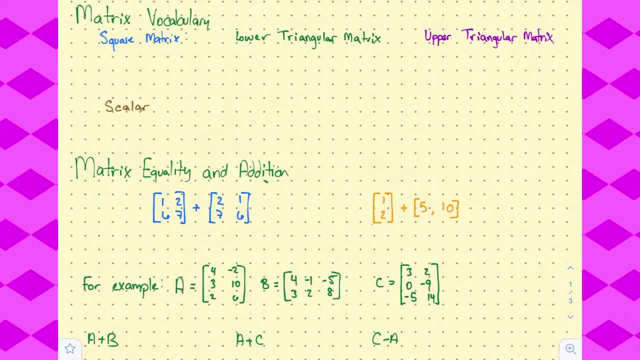 Square matrices, or a square matrix is a matrix that has the same number of rows and columns. They can be in any size. So here's a 1 by 1 square matrix. Here's a 2 by 2 square matrix. 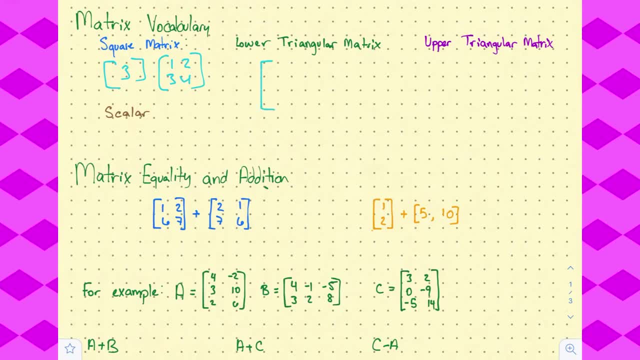 Triangular matrices are a special case of square matrix. The matrix itself is not shaped like a triangle, but the data inside is The term upper or lower matrix. is a square matrix Than that, the Midwestría matrix is spelled out as the lower matrix for the unconscious. 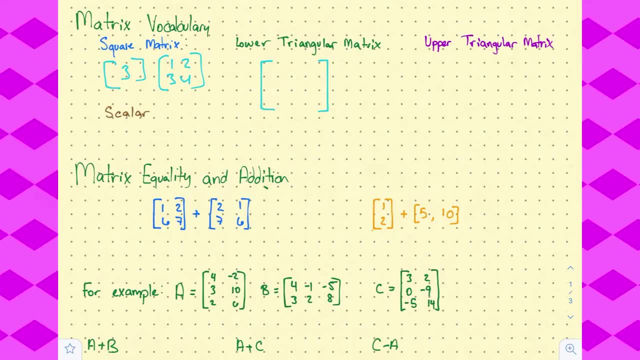 Lord. So this bottom right is a square matrix, Then the bottom lower just refers to where the data is. So a lower triangular matrix is a square matrix, but everything above this main diagonal is just going to be a 0. Just filler space. 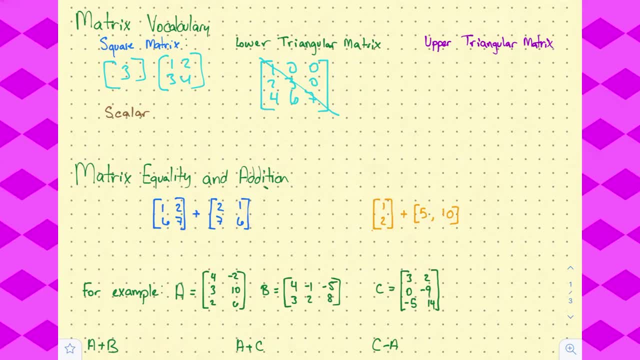 Whereas our actual information filers in everything on or below that main diagonal. Plus there is another higher event. Most of the times we just lined this off and have a d2学 2.. It's the same thing, ira, So that's a lower square matrix. 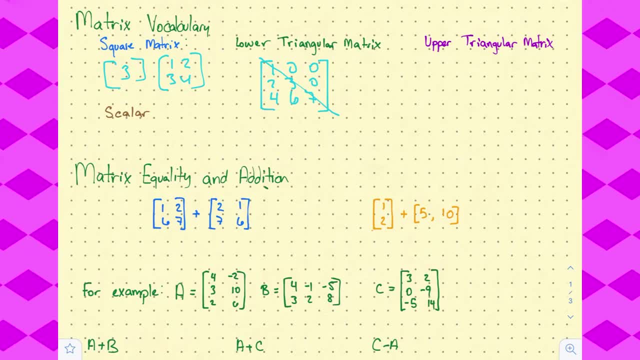 So that's a lower triangular matrix. An upper triangular matrix is just the reverse, where the data is all on or above that main diagonal and its zeros below. Now, a scalar is just a fancy word for a number, Since we're dealing with two-dimensional arrays of numbers. a scalar just refers to a one-dimensional array. 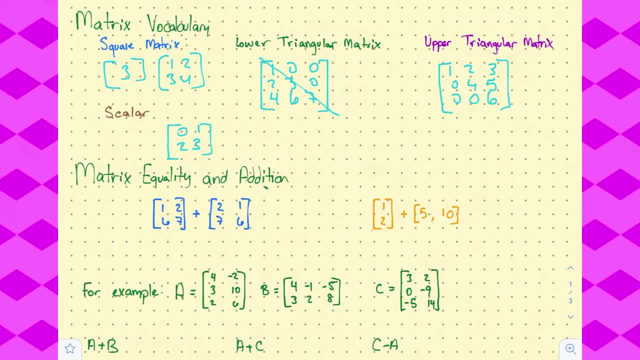 We use scalars when we do repeated addition or we can multiply matrices by a scalar. A scalar in this context just refers to a number. Now it's important to talk about what it means when we say two matrices are equal. Now it might sound intuitive. 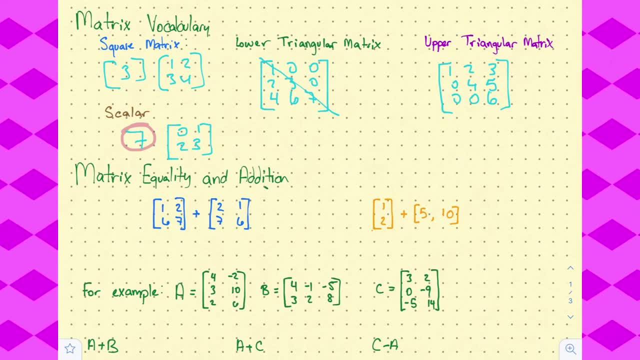 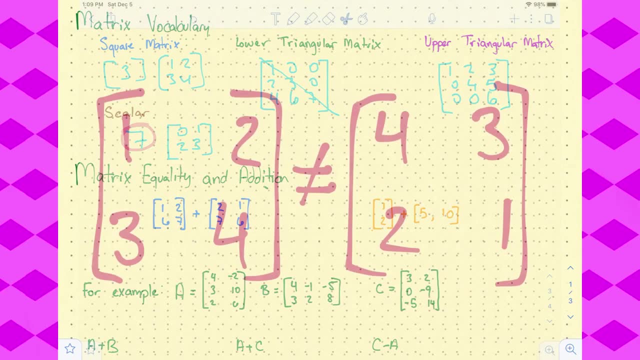 But it's important to note that two matrices are only equal if they have the same elements in the same location. So the array 1, 2, 3, 4 is not equal to the array 4, 3, 2, 1.. 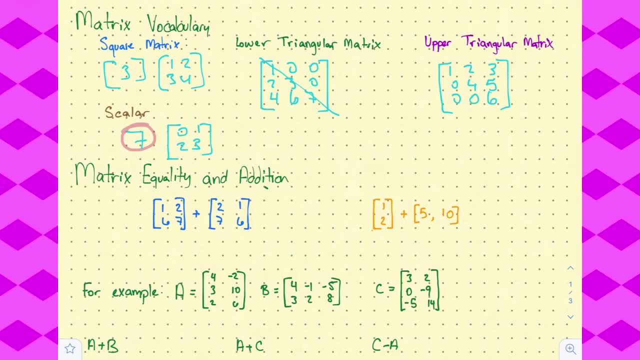 You might have been able to figure that out on your own. I just wanted to make sure that we said that out loud. So now that we know what a matrix is, now that we know what it means for two matrices to be equal, we should probably be able to do some basic operations with arithmetic. 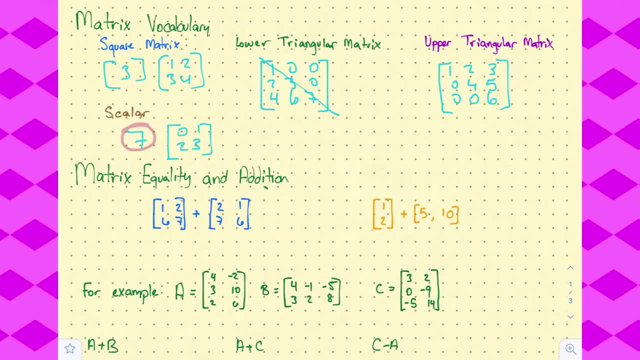 So let's start with addition. To add two matrices, you just add the corresponding elements. So this matrix, I just need to add the 1 and the 2,, which is 3, the 2 and the 1,, which is 3,. 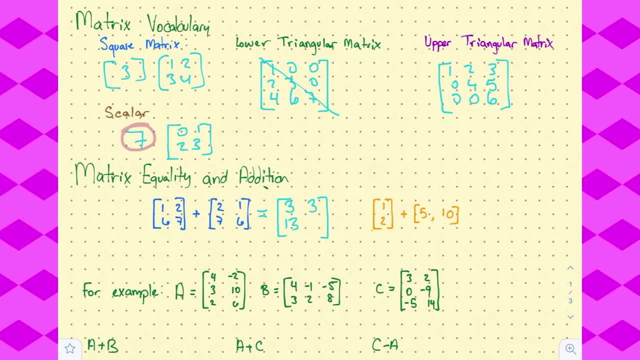 the 6 and the 7,, which is 13,, the 7 and the 6,, which is 13.. Now, one very important thing to pay attention to are the dimensions of each matrix, Because we have to add the corresponding elements. 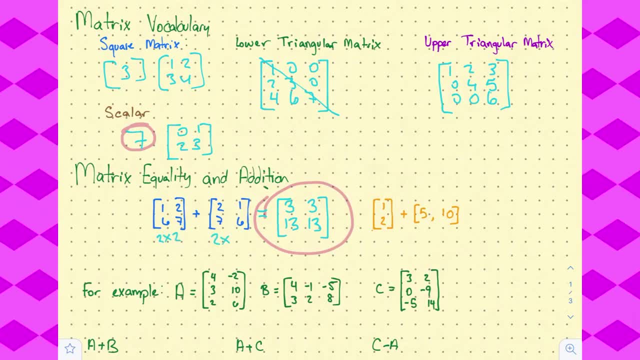 if the dimensions don't match up, I cannot add them. So for this next example, we see this is a 2 by 1 matrix and I'm trying to add it to a 1 by 2 matrix, While I might be able to add the 1 and the 5,. 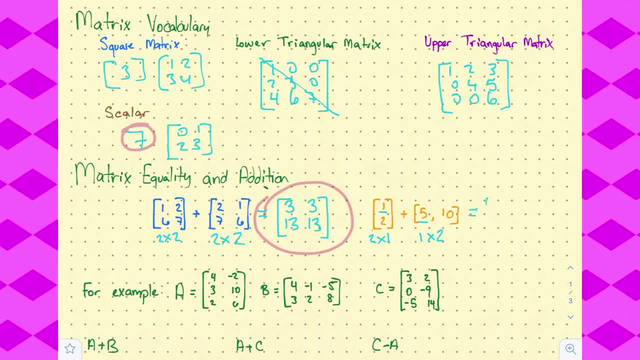 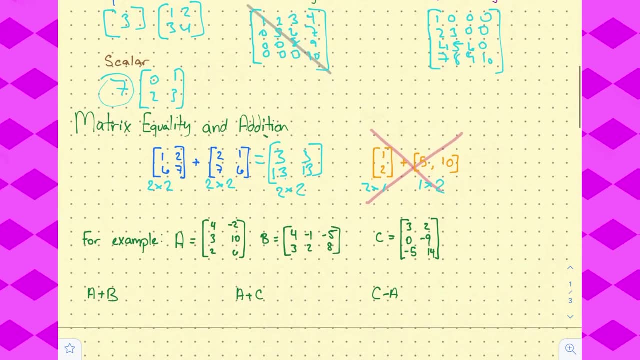 I don't necessarily have anything to add the 10 to or the 2, and I'd be left with this blank space down in the bottom corner. So we just say that we cannot add those two matrices. So let's check out another couple of examples. 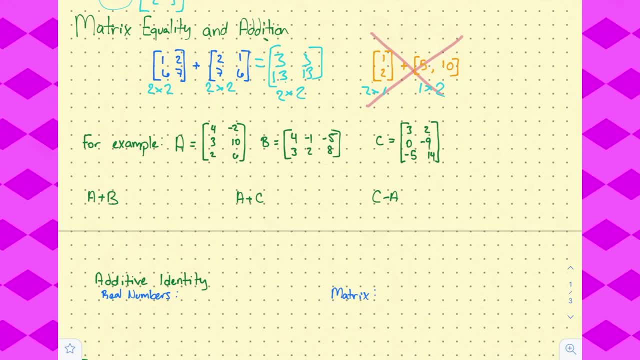 a plus b. a is a 3 by 2 matrix. b is a 2 by 3 matrix. This one is not possible. However, I can add a and c. To add a and c, because they are both 3 by 2 matrices. 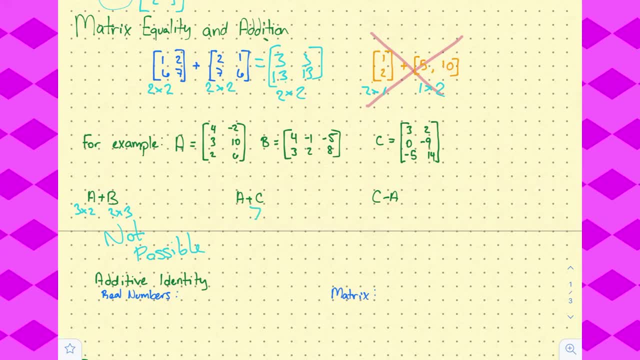 I just need to add their corresponding elements: 4 plus 3 is 7.. Negative: 2 plus 2 is 0.. 3 plus 0 is 3.. 10 plus negative: 9 is 1.. 2 plus negative: 5 is negative 3.. 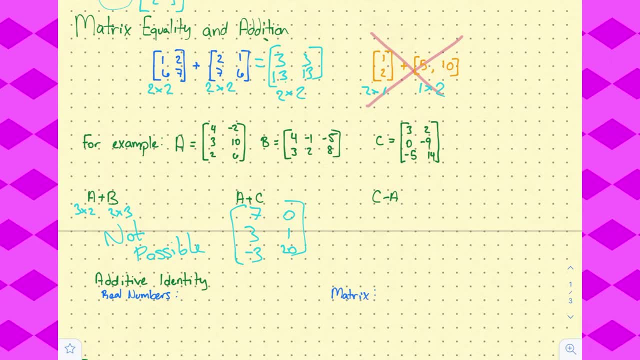 And 6 plus 14 is 20.. And c minus a works the same way. I'm going to subtract my corresponding elements: 3 minus 4 is negative 1.. 2 minus negative 2 is 4.. 0 minus 3 is negative 3.. 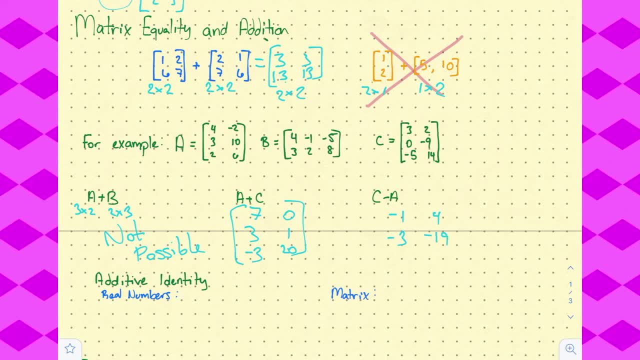 Negative 9 minus 10 is negative 19.. Negative 5 minus 2 is negative 3.. Negative 7 plus 14 minus 6 is 8.. So to add or subtract, you just add or subtract the corresponding element. This brings me to my next idea, the notion of an additive identity. 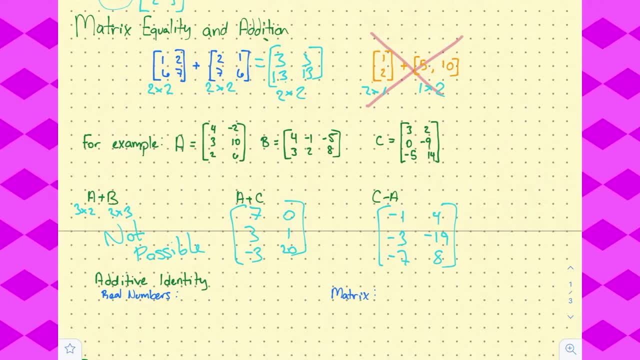 The term additive identity just means something you can add without changing its value. In the real numbers, that number is 0. If you ever add 0, that does not change the value For matrices. the additive identity is just the 0 matrix. 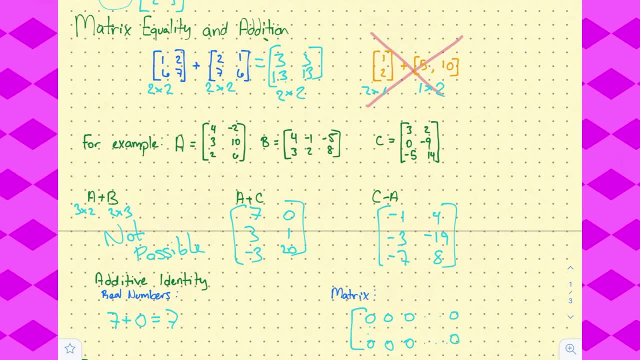 It's as big as you need it to be, so that the dimensions match, But it's filled with 0s. That way, when you add it to another matrix, the dimensions do not change. We call this matrix O, So for any matrix. 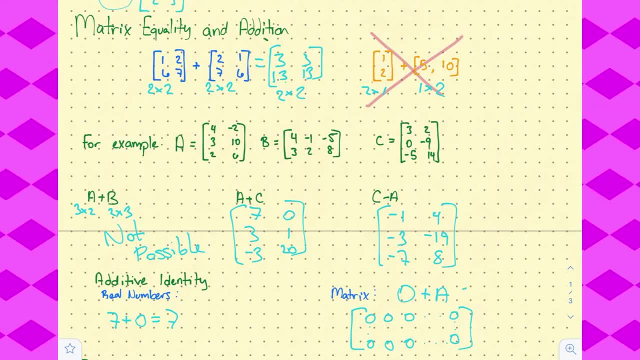 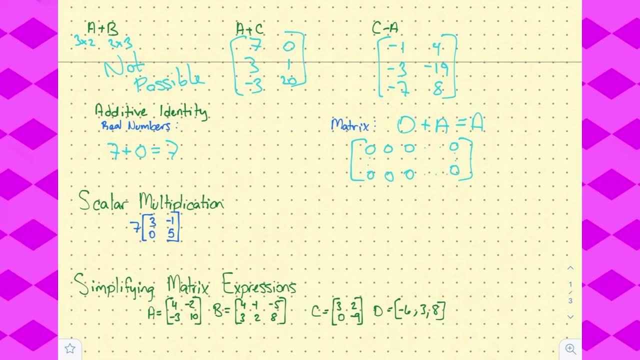 for any matrix, A, O plus A is equal to A. Another idea we need to be able to do is scalar multiplication. So I noted earlier that a scalar is just another word for a number. So scalar multiplication is just multiplying a matrix by a number. 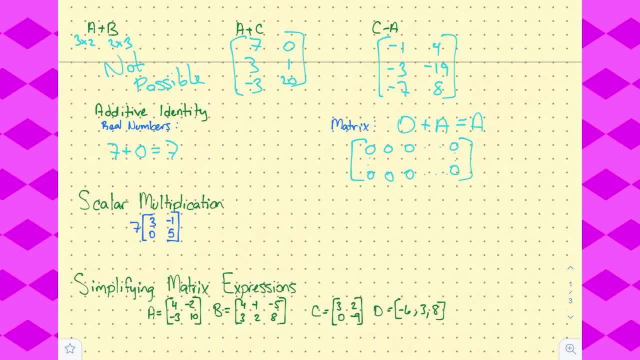 This idea follows straight from our notion of multiplication in real numbers, where it's just repeated: addition 7 multiplied by the matrix 3, negative 1,, 0,, 5, is the same as adding that matrix to itself 7 times. 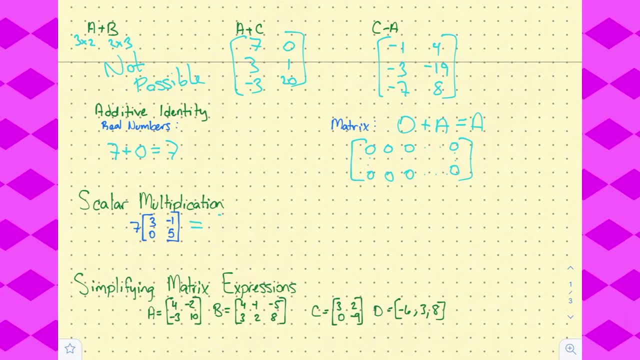 So to do the scalar multiplication you just need to distribute 7 times 3,, 7 times 0,, 7 times negative 1, and 7 times 5.. Multiplying two matrices together is a little more complex. We'll save that for a future lesson. 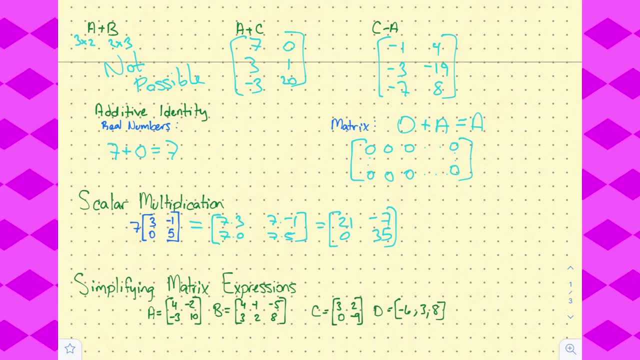 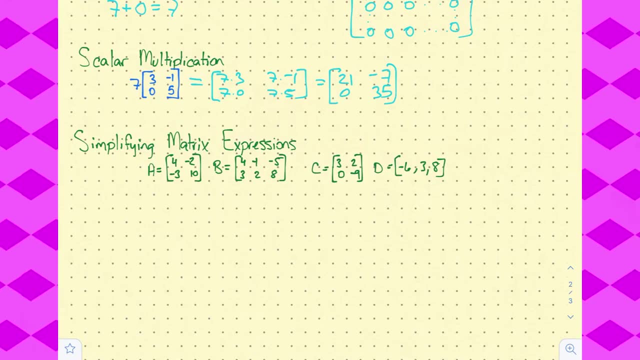 So now that we've talked about how to add and subtract and multiply a matrix by a scalar, let's look at a matrix expression we should be able to simplify. So here are four matrices I'd like to evaluate: 2A minus 3B. 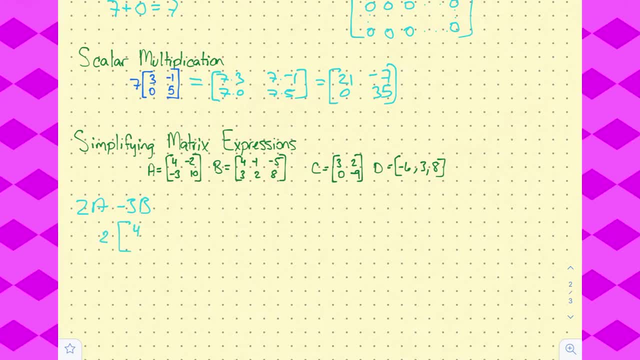 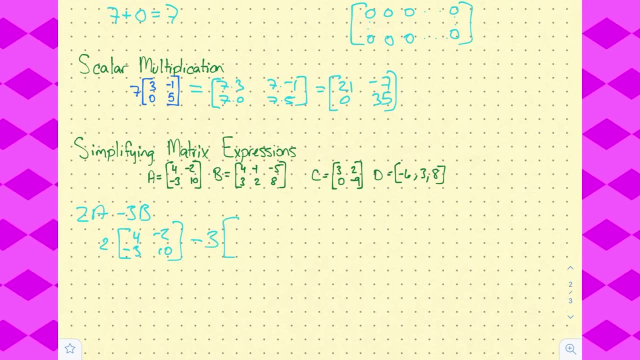 So 2A minus 3B is 2 multiplied by the matrix 4, negative 2, negative 3, 10, minus 3 times the matrix 4, negative 1, negative 5, 3, 2, 8.. 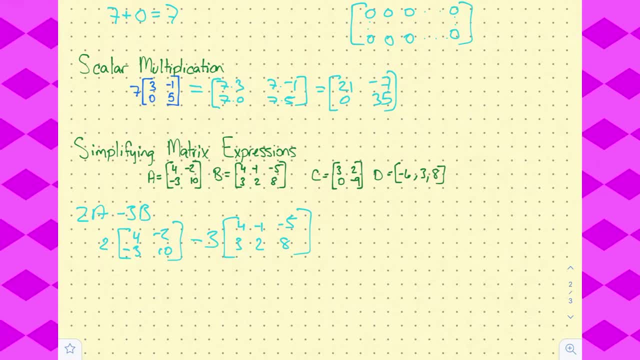 Now let's check out the dimensions and what's going to happen. 2A is going to be a 2 by 2 matrix, whereas 3B is a 2 by 3 matrix. Our dimensions don't match, so I cannot do this addition.